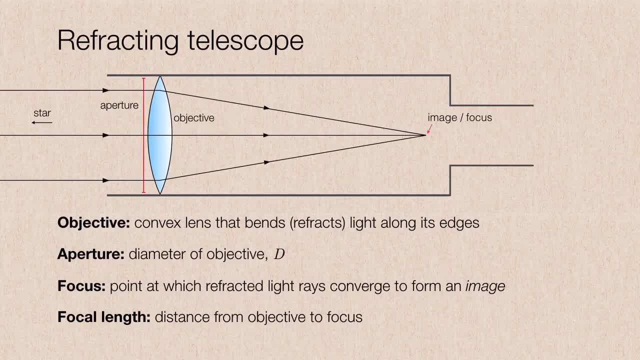 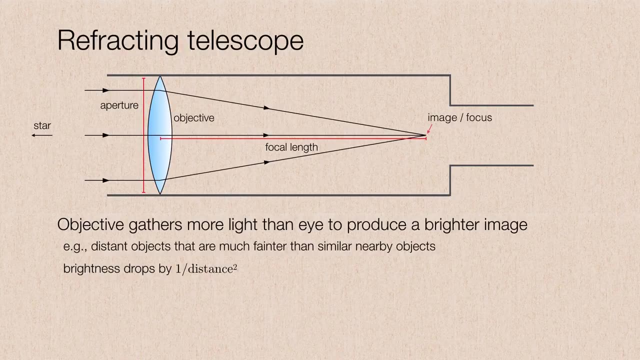 to form an image, And the point at which it forms the image is called the focus. Therefore, the distance from the objective to the focus is called the focal length. So what is the purpose of the objective? Well, it's simply to capture more light than the eye can produce and therefore, 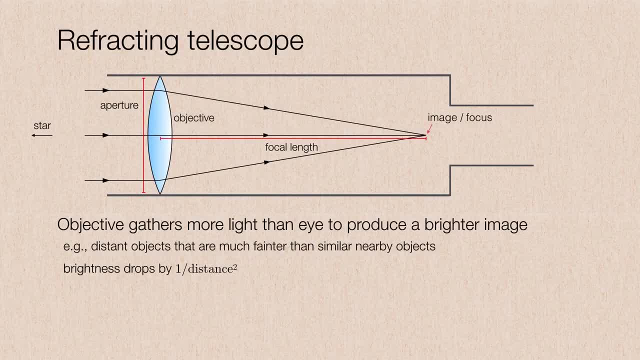 producing a brighter image. Now, we've already shown that brightness drops by one over the distance squared, So the more distant an object is, the fainter it's going to be. Therefore, the larger aperture objective can gather that much more light and form a brighter image. And 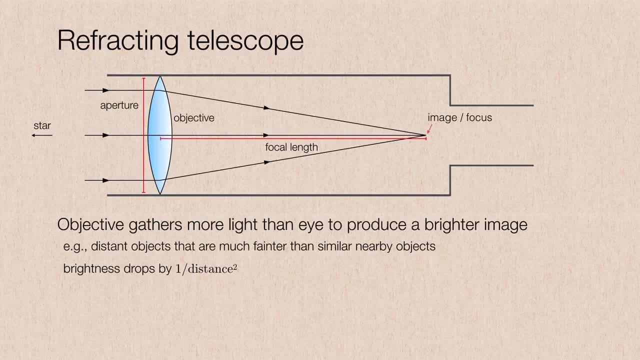 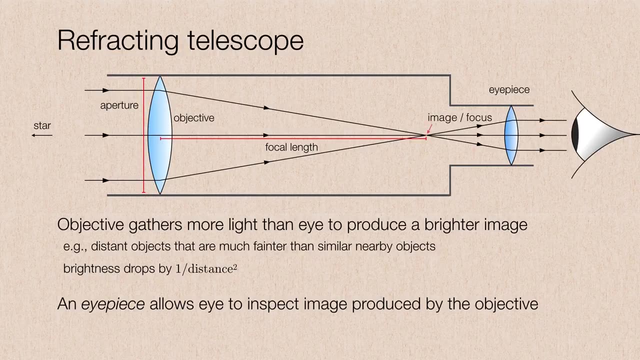 this is particularly useful for stars, which are very dim compared to everyday objects that we look at during the daytime. Now, in order to inspect this image, we need to employ a second lens. This is commonly known as an eyepiece- And what this does is it lets the light rays. 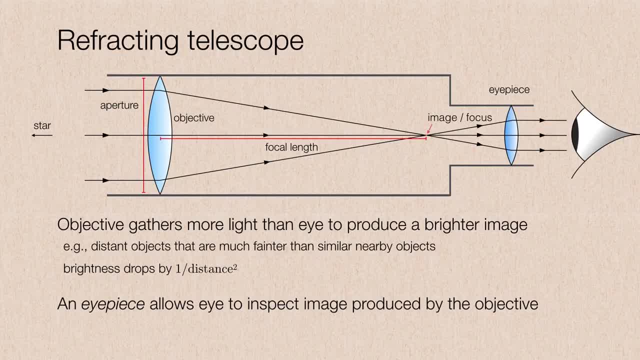 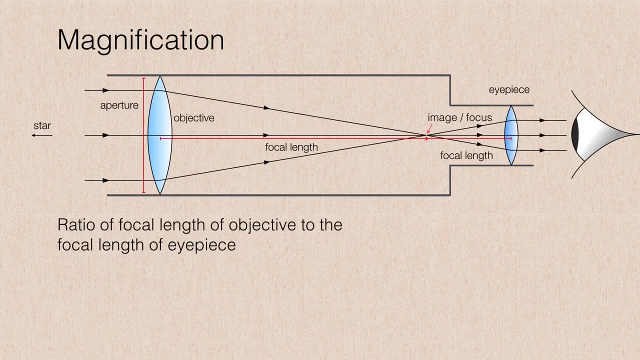 spread apart once again and then focuses them into an image. So it basically magnifies the image and allows the eye to actually see the image produced by the objective. So the eyepiece is also going to have its own focal length And therefore the ratio of the two focal. 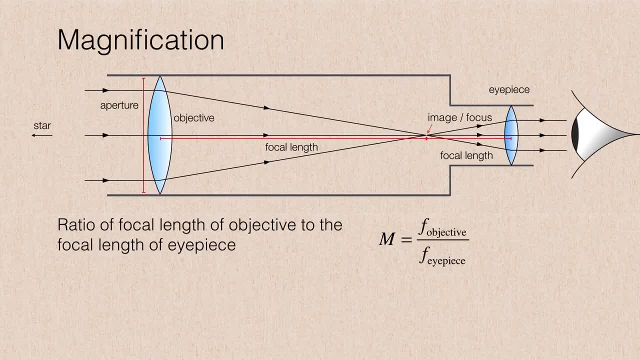 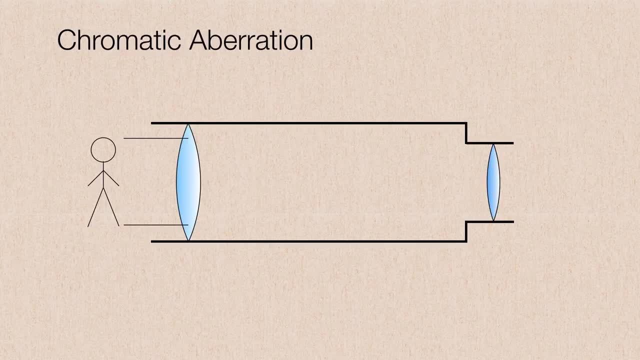 lengths. the ratio of the objective's focal length to the eyepiece's focal length is what we refer to as the magnification. Now, if you think about the way light behaves when it passes through any medium, it typically will disperse into its component colors And the same effect happens. 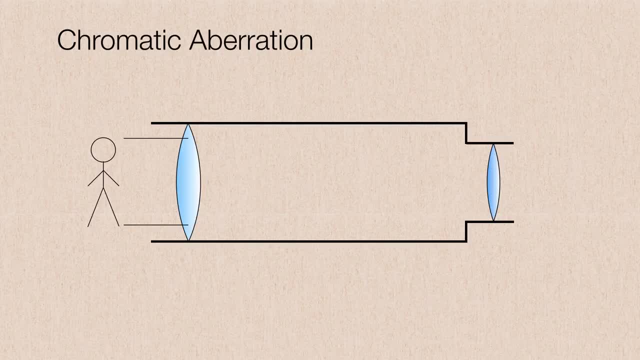 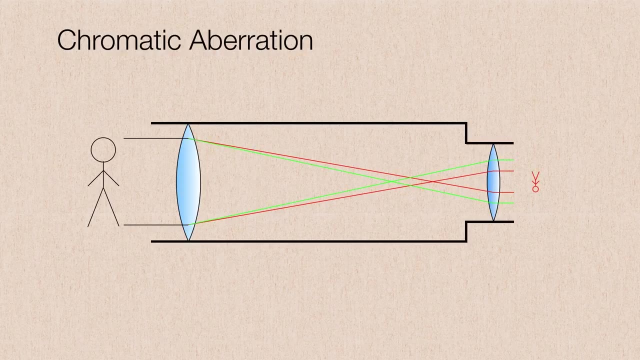 here. So here's a really simple or oversimplified version of looking at somebody through a refracting telescope. So light rays are going to reflect off of the individual and they're going to pass through the objective, But in so doing they are refracted by different amounts, And so 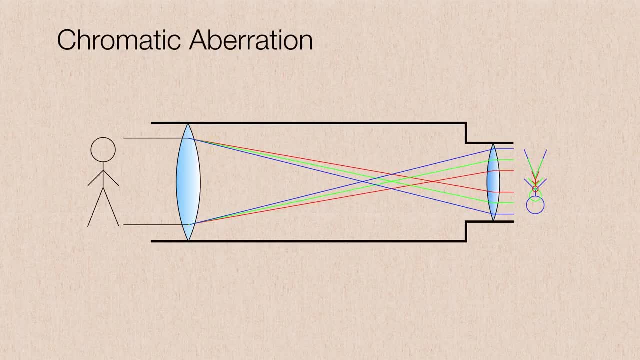 different colors form images at different focal lengths from the objective. But it's even worse than that, because you can't focus on all three of these images simultaneously. You have to pick one color and then let the rest just blur out. So this is a phenomenon known as chromatic aberration. 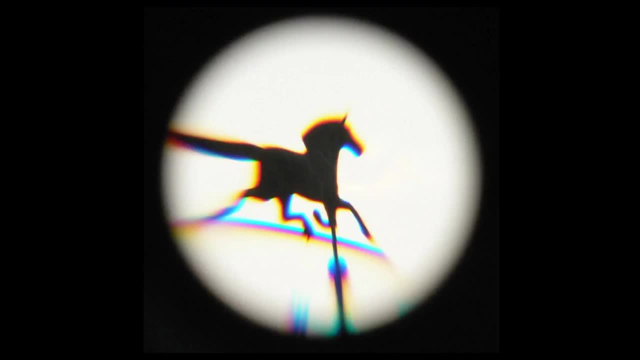 and if you ever use a lens that does not have any corrective elements in it, then you're going to see this effect in action. So here's a weather vane. We can see colors just spilling everywhere. In order to fix this problem, most refracting telescopes are: 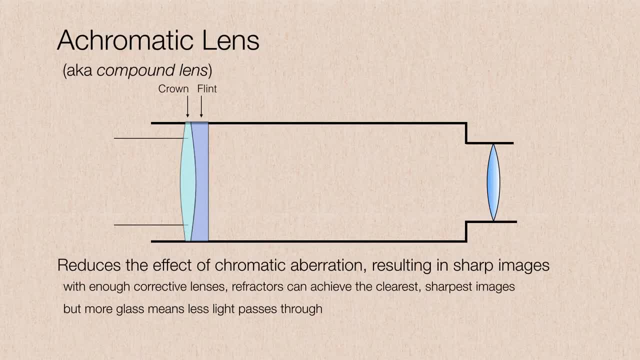 fitted with what are called achromatic lenses, or sometimes called compound lenses. Simply, they introduce a secondņ lens element that has the effect of re-bending or re-refracting the shorter wavelength light, such that all the focal lengths of all of the different 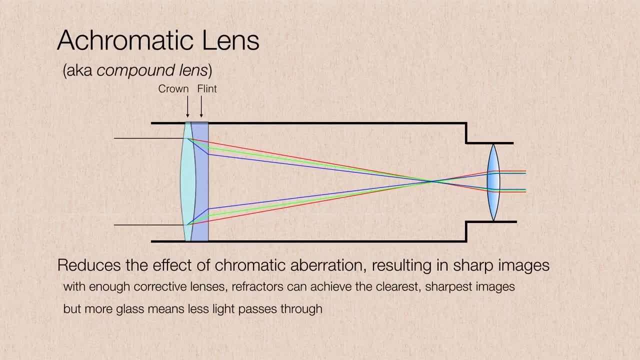 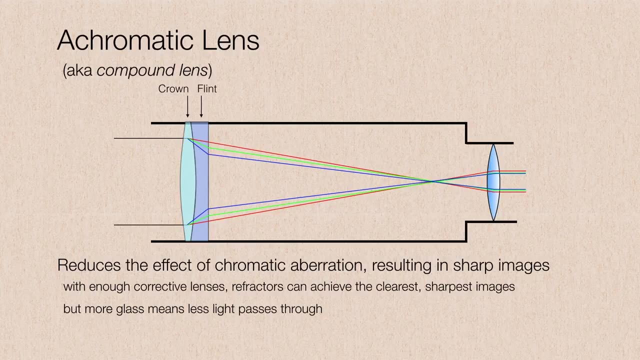 component colors of light converge once again, forming a nice, clear image. In fact, you can obtain the sharpest images this way. However, we are employing more glass to produce the image, and every time you let light pass through some glass, you're going to lose a few photons here and there. So, depending upon your application, 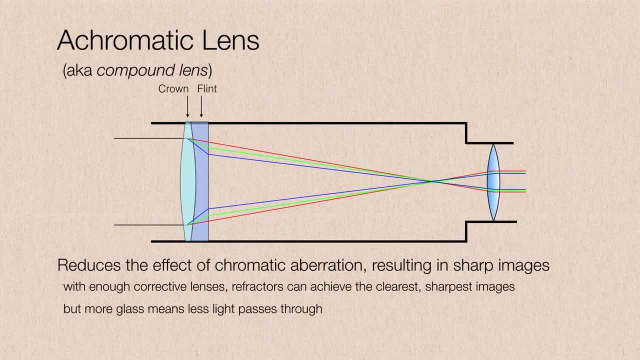 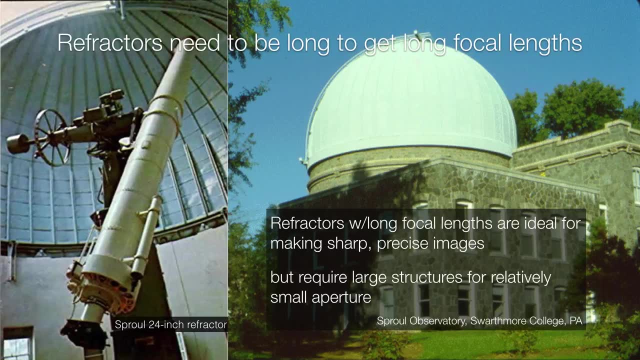 you may or may not want to lose those extra photons. Still you can get the sharpest images this way. In fact, I got to use a telescope of this very same configuration when I was working at the Sproul Observatory at Swarthmore College. 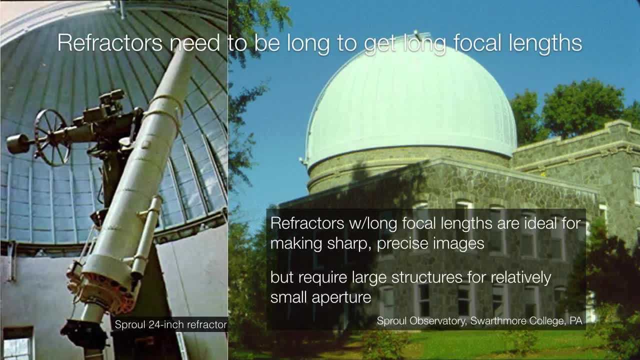 back when I was a kid. You can see here just how big the observatory that the enclosure needs to be in order to accommodate the light that's coming in and out of the observatory. You can see here just how big the observatory that the enclosure needs to be in order to accommodate. 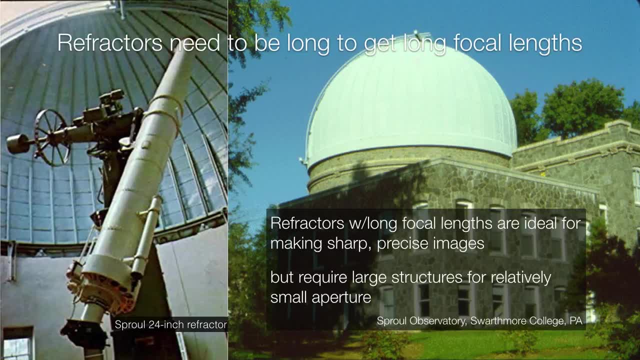 this telescope. This telescope has an aperture of 24 inches, about two feet, which is, by today's standards, not very large for an astronomical telescope. and yet, despite having a rather modest aperture, it had to be enclosed in a building that had more cubic volume than the house I grew up in. So here we have a. 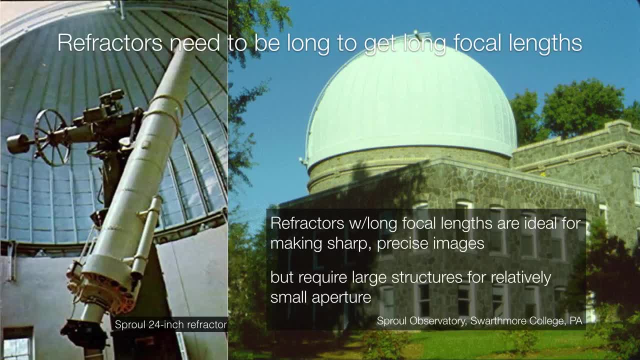 telescope with a rather long focal length and we don't have any way of short cutting that focal length. It needs to travel all the way through that tube in order to come to a focus before it goes into the camera at the bottom of the picture. So you are stuck with a very large building to accommodate a rather 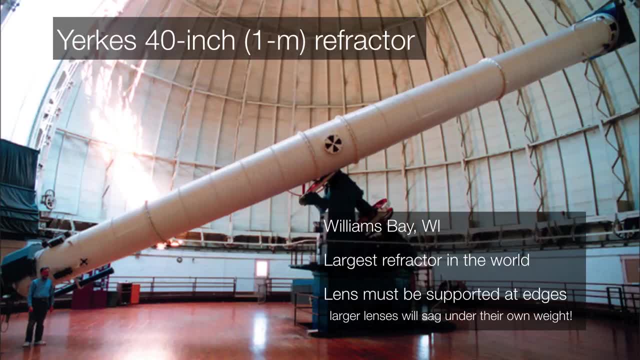 modest sized refracting telescope. Remember, these lenses have to be supported by their edges, therefore you can't put anything behind the lens to keep it upright, or else you're gonna block light. So anything beyond about a meter in diameter and the lens will start to just sag underneath its own weight and become useless. 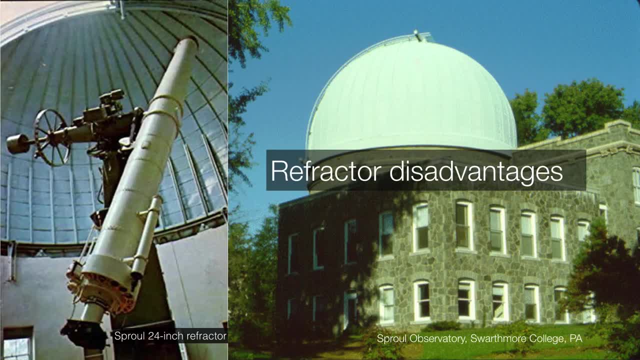 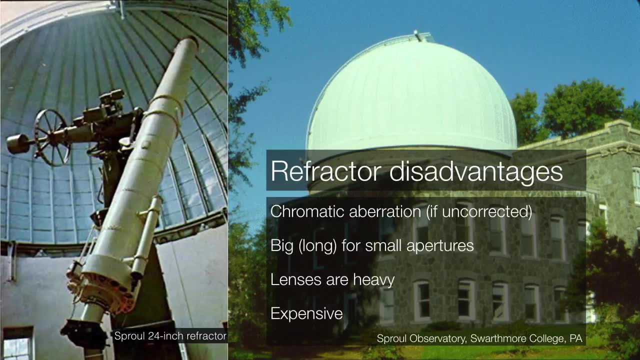 So refracting telescopes have several fundamental disadvantages, not the least of which is chromatic aberration. Then you have to build them very long for modest apertures. That in turn requires very large structures in order to house them. The lenses are very heavy and they are very difficult and therefore very 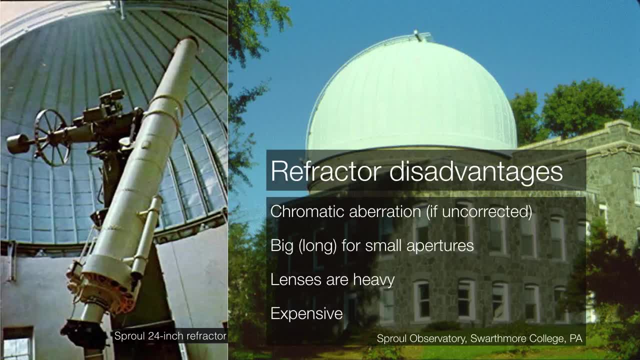 expensive to produce Now. the problems with refractors were well known as far back as Isaac Newton's time, and Newton himself developed a very complex system of refractors. The problem with refractors is that they are very difficult and therefore very expensive to produce. Now. the problems with refractors were well known as far back as Isaac Newton's time, and Newton himself developed a. 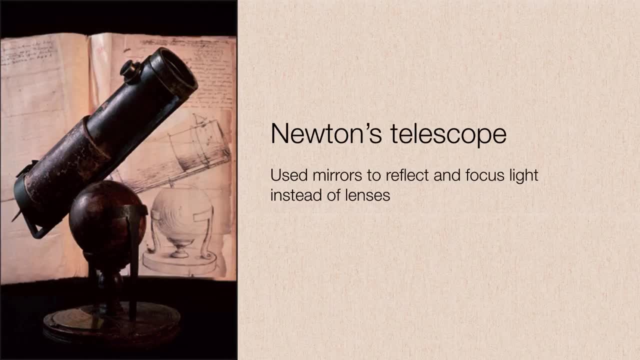 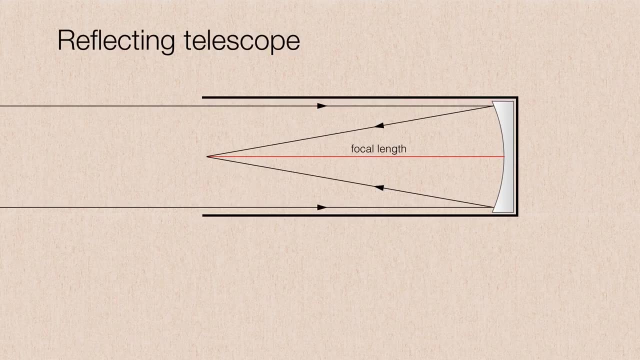 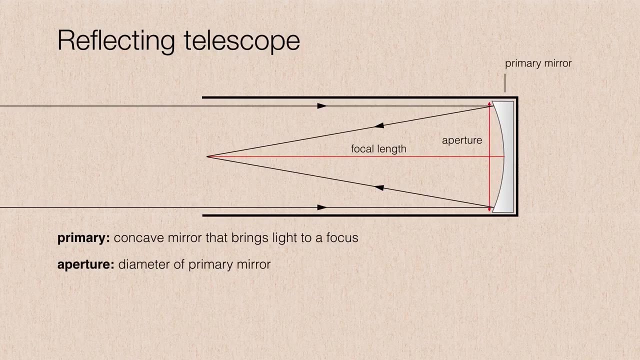 alternative method of building telescopes, this time using mirrors instead of lenses, And so the reflecting telescope operates this way: There is a primary mirror and, just like we saw with the refracting telescope, its diameter is the aperture, So the light reflects off of the primary mirror. You notice that the 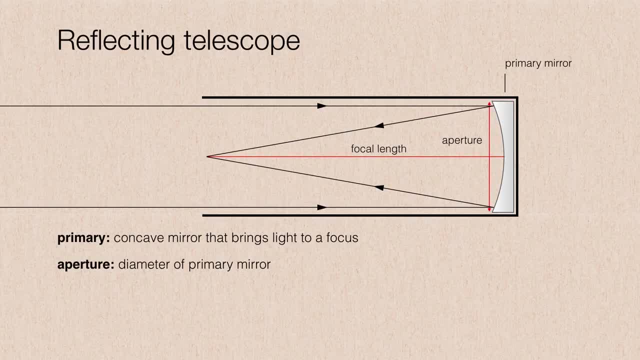 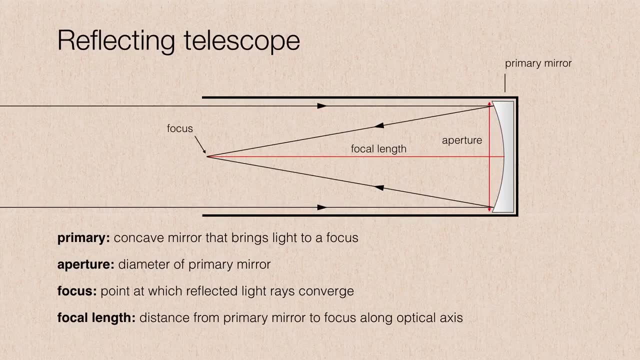 primary mirror is concave in shape. This allows the light to come to a focus, and at this point we could make an image, Except for one problem, and that is, if we were to place our eyes there, then the rest of our head will block out the incoming light. So what Newton did, is he? 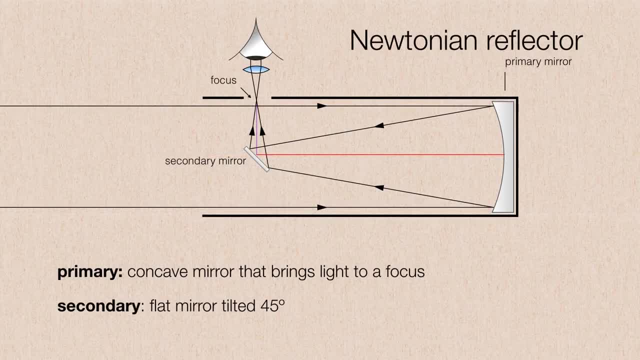 just set up a 45 degree mirror, called a secondary mirror, and redirected the light out the side of the telescope's tube, Place an eyepiece there and now you have a nice focused image. and now you're not blocking out any light- A problem. 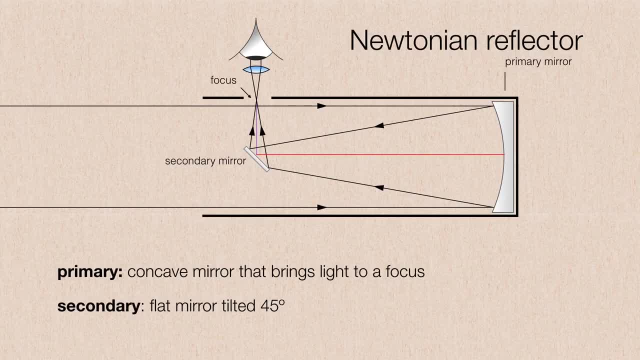 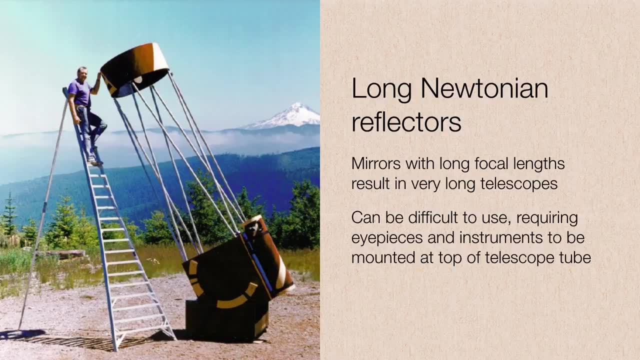 with Newtonian reflecting telescopes, though, if you're going to build a telescope with this particular configuration, is that you may be running into a potential safety hazard if you built a telescope with a long focal length mirror, So you got to be a little careful in situations like this. There's an alternative configuration that astronomers like 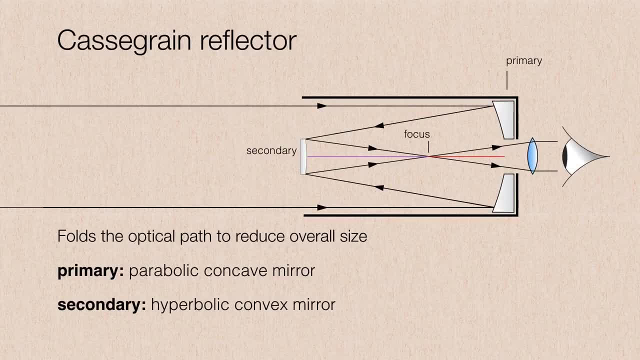 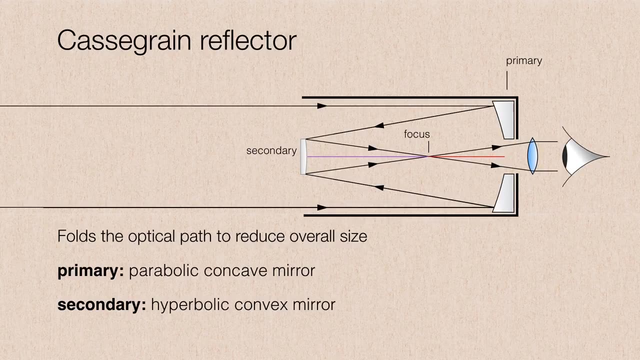 to use, and it's called the Cassegrain reflector. So, rather than use a 45 degree flat mirror, a secondary mirror is set up that is convex in shape, And what this does is it redirects the light out through a donut hole cut in the back of the primary mirror. Now this donut hole does 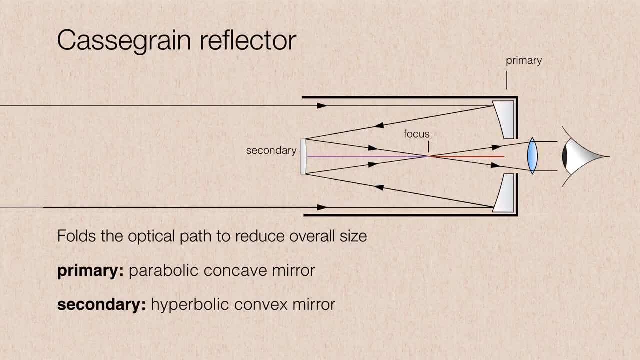 mean that we're going to lose some of the light, but this also means that the telescope's focal length effectively gets folded up into thirds, So we can have a telescope that is much more compact, even though it could have a potentially nice long focal length. 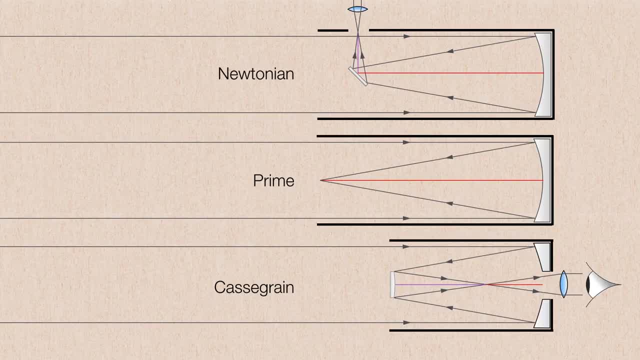 So there are three main types of reflecting telescopes. There is the Newtonian design that we talked about before. There's also the prime telescope or the prime focus telescope. If you can get a camera small enough relative to the mirror, you could fit it there at the prime focus.